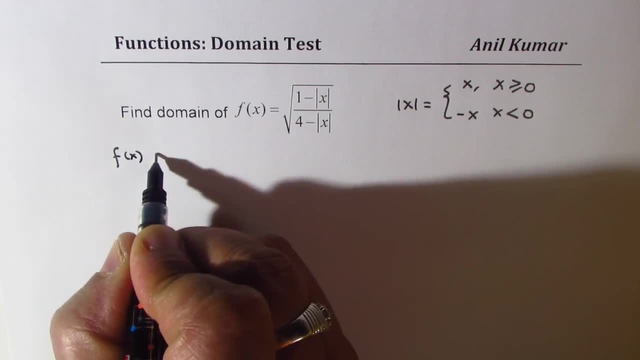 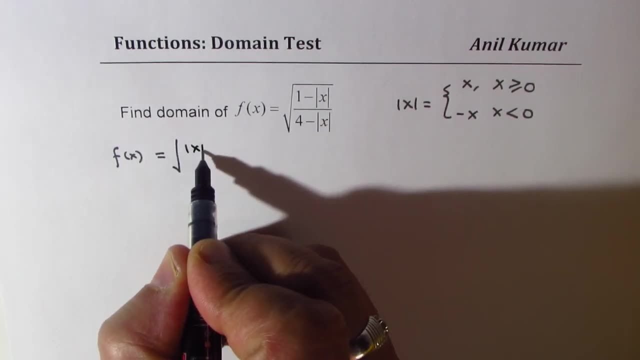 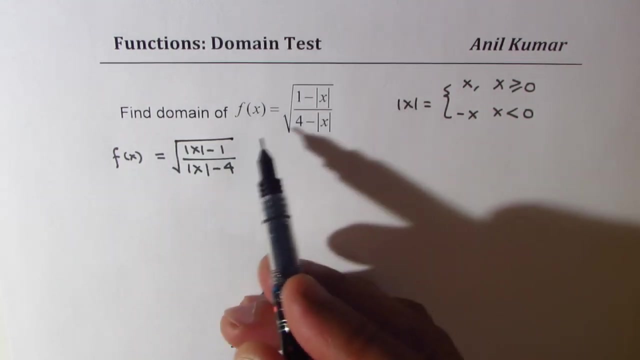 Now I could also write this function f of x as equal to. I mean, both could be negative outside, so it is as good as writing absolute x minus 1 over absolute x. Absolute x minus 4, correct, It is same as what is given. Now let us divide this page. 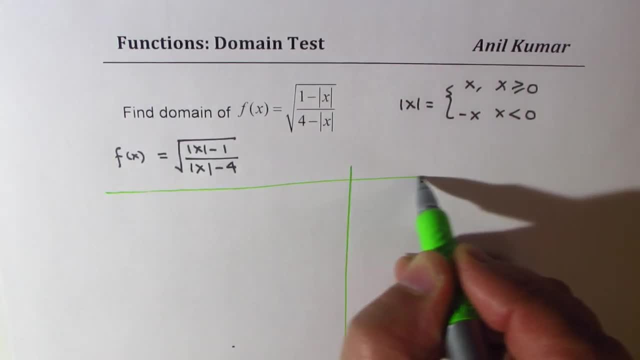 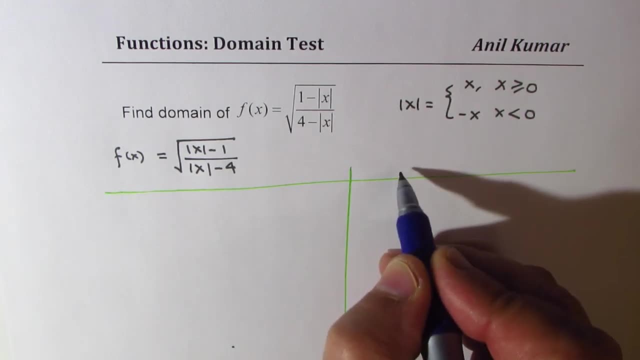 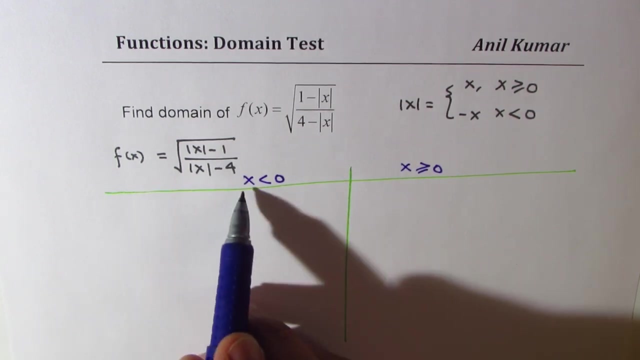 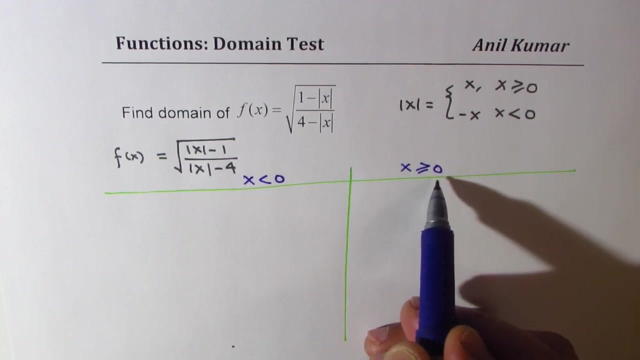 into two parts and solve the question for two different intervals: One when x is greater than or equal to 0,. the other one when x is less than 0,. right Now, if x is less than 0, then absolute x will be replaced by minus x, and when x is greater than or equal to 0,. 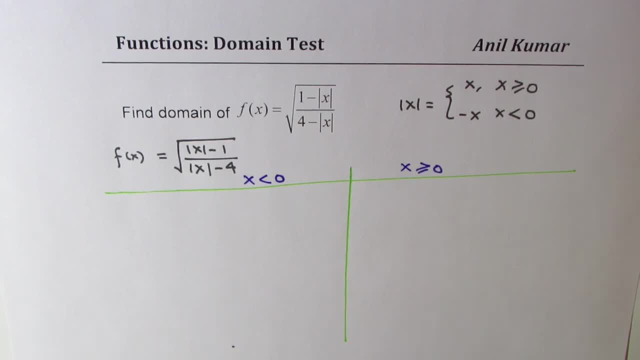 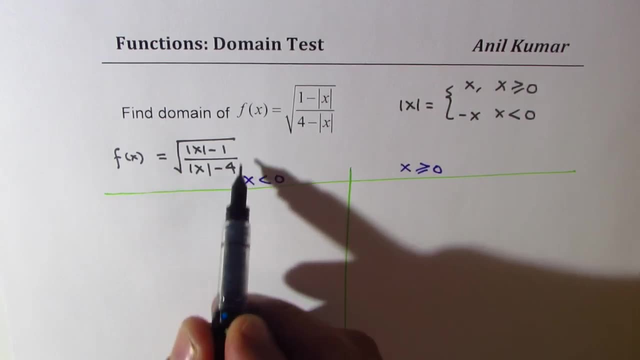 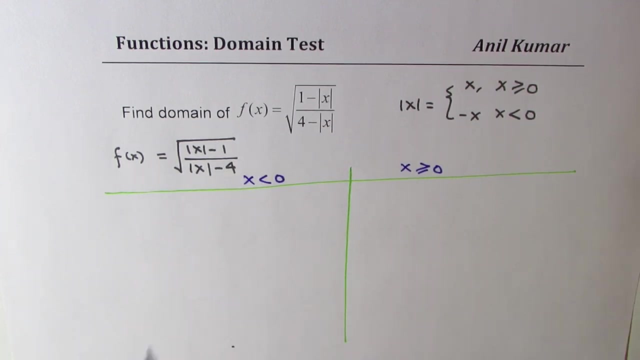 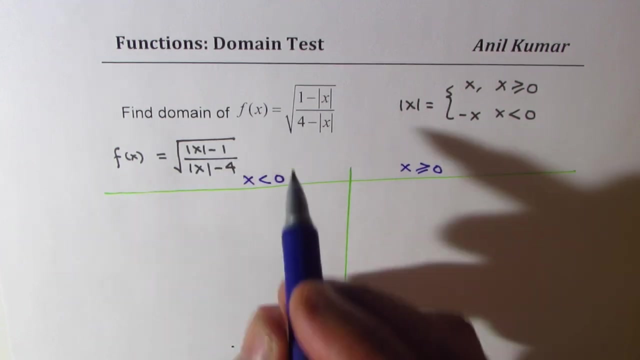 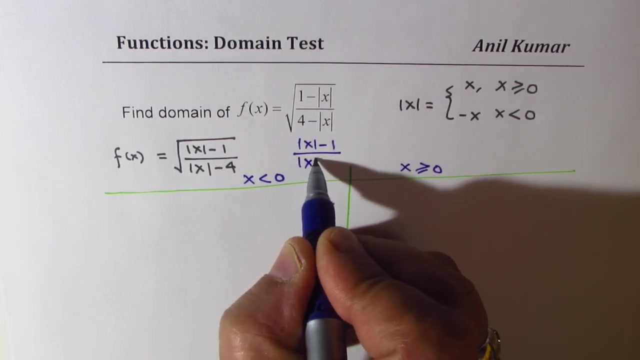 absolute x will be replaced by positive x, correct? So then what we get here is this particular function. But see, when we are talking about domain, we also want that within the square root, everything is non-negative. That is to say, we want absolute value of x minus 1 over absolute value of x minus 4. 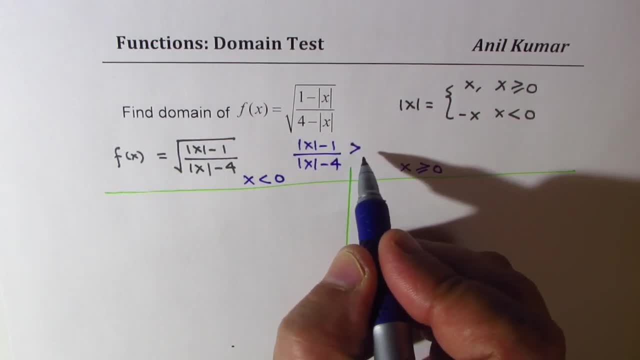 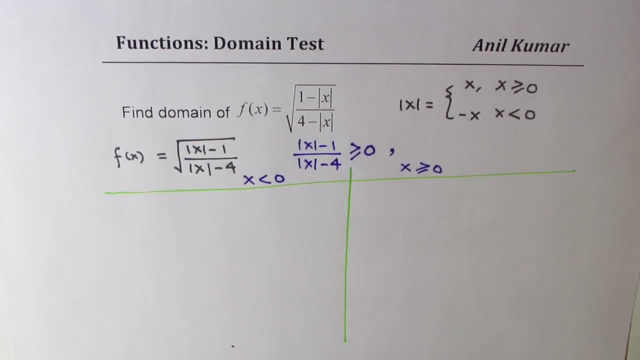 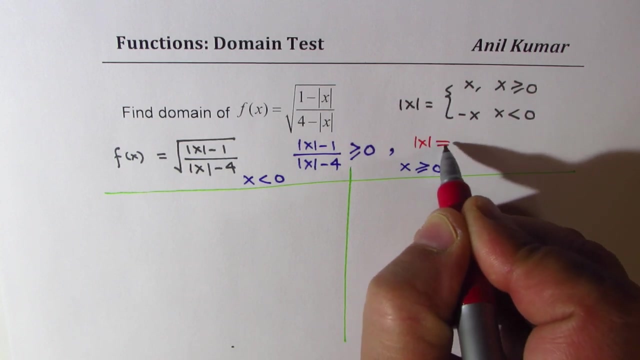 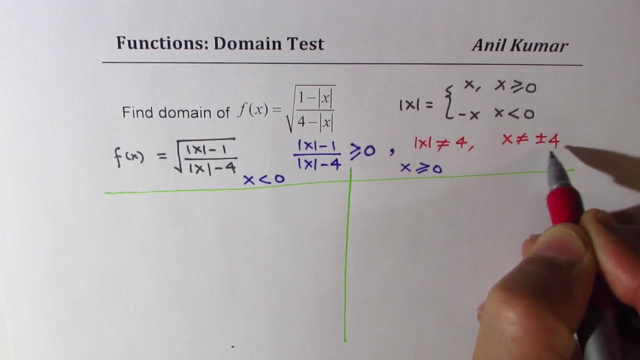 should be greater than or even equal to 0, right Now, denominator cannot be 0. So that gives us one restriction which is absolute: x is not equal to 4.. So gives you that x is not equal to plus minus 4.. So that is one part of our solution. Now we have 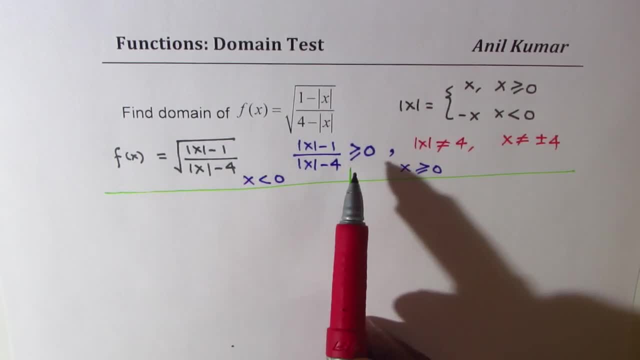 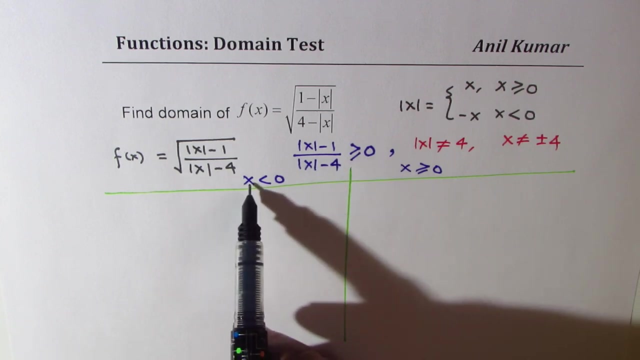 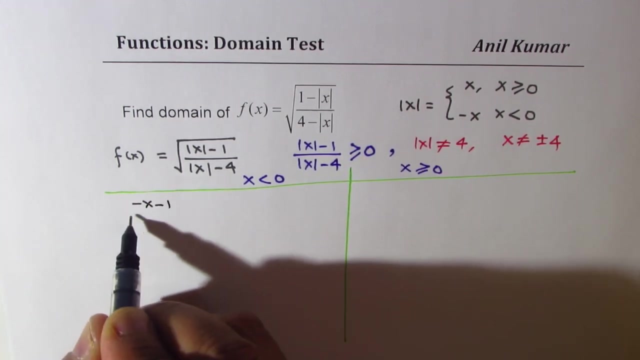 to see the interval where the whole function is non-negative. It could be 0.. It is valid at 1,, for example. right, Okay, So basically you are looking into this part Now. when x is less than 0, absolute x will be written as negative x, So we'll replace it with negative x, negative 1,. 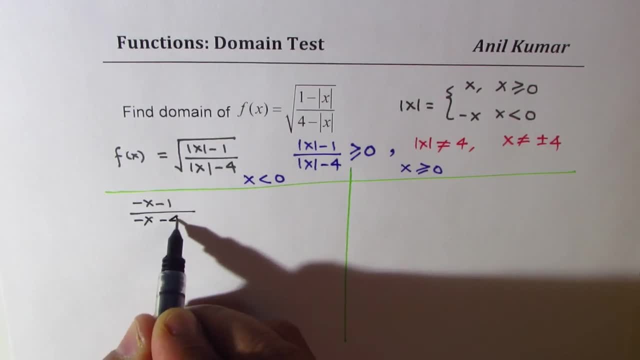 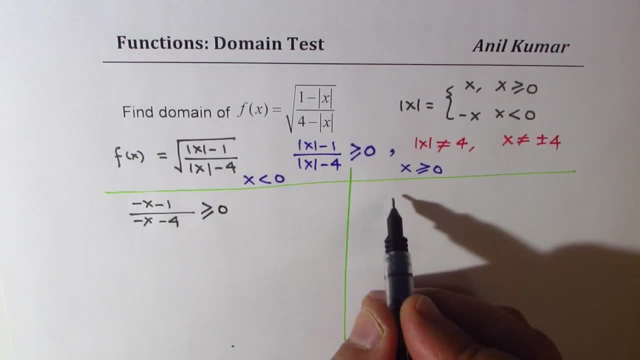 negative x for absolute x. correct. And the inequality. we want to show that this should be greater than equal to 0. Here, when x is greater than 0, absolute x is positive x. so we get x minus 1 over x minus 4 greater than equal to 0, correct. 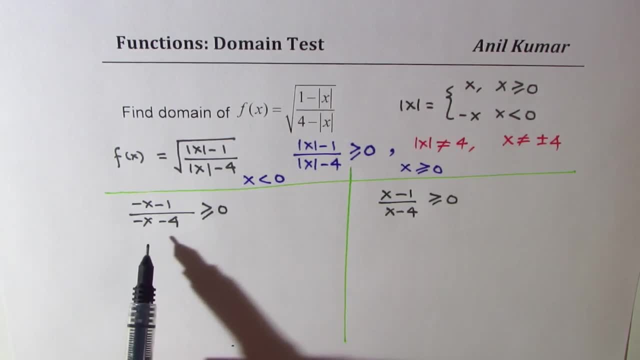 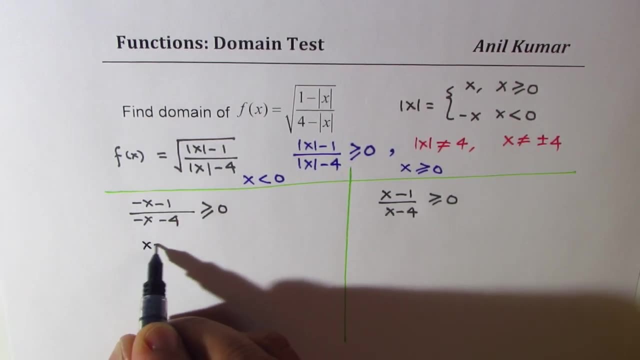 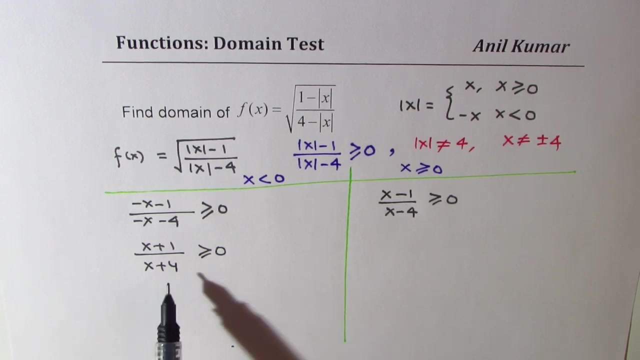 Now, when is this greater than equal to 0?? We could take minus common. Let me rewrite this as x plus 1 over x plus 4 greater than equal to 0. This is better. Now there are two intervals which we have to look into when we solve this question. Let's do it here. 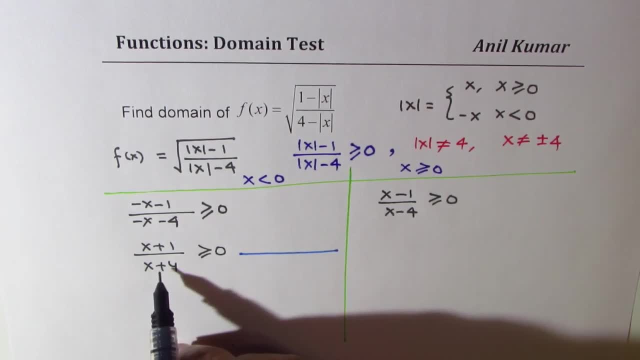 We know that it is at minus 4 and minus 1.. At minus 4, we'll have a vertical asymptote, kind right. So this is at minus 4.. And then at minus 1, we could have a 0. So that will work for us. 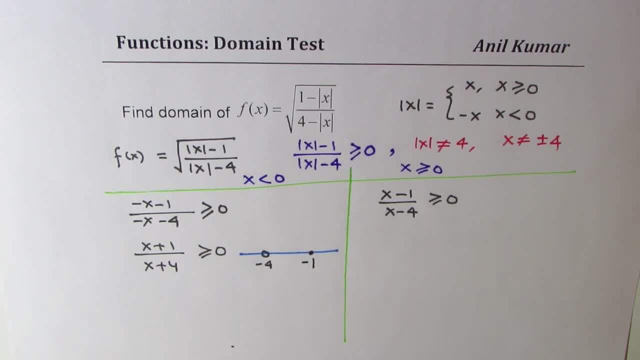 We have to analyze this within these three intervals. So let's take test points. On the left side it will be minus 5.. Here we could take minus 2.. And we can take, let's say, minus half, here 0.5.. If I substitute minus 5 here, both become negative. And what we 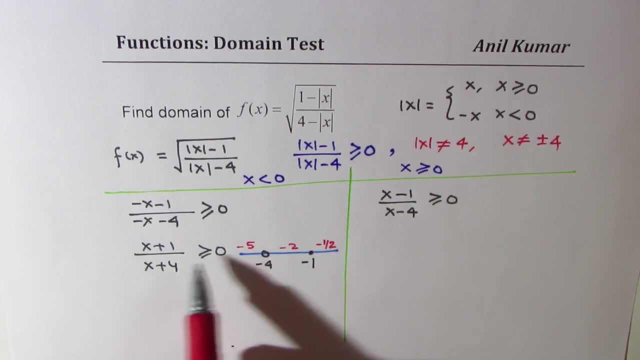 get here is that it is actually positive, right? So if I do minus 5, we get minus 4 over minus 1.. So this is positive here. If I substitute minus 2, numerator is negative. However, denominator is positive. That gives me negative result. And for minus. 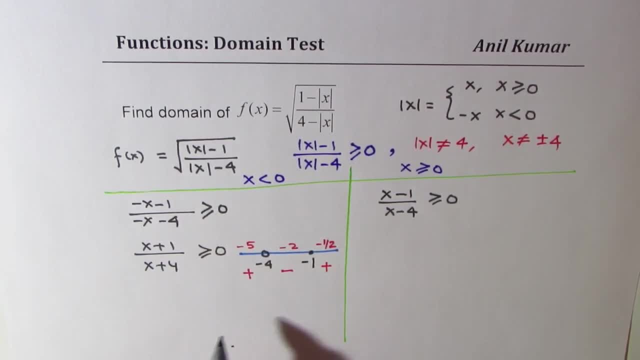 half, both are positive. So this inequality greater than works in these intervals, which is x could be less than minus 4, or x could be greater than minus 1, right, Greater than equal. to Remember, x is within this. So 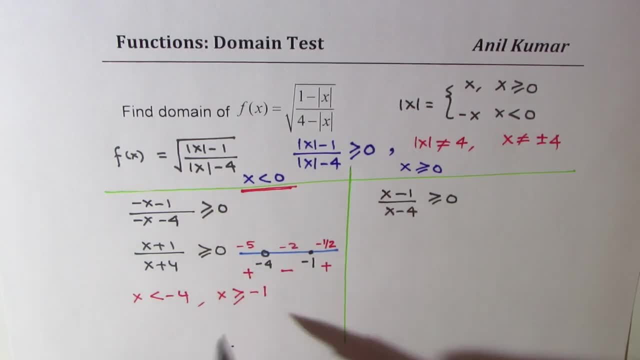 since we have this condition here, we should rewrite this as x is less than minus 4.. That's perfect, But x is greater than equal to minus 1, but less than 0, correct, Since that is the interval in which we are working. So that becomes the solution from the left side.